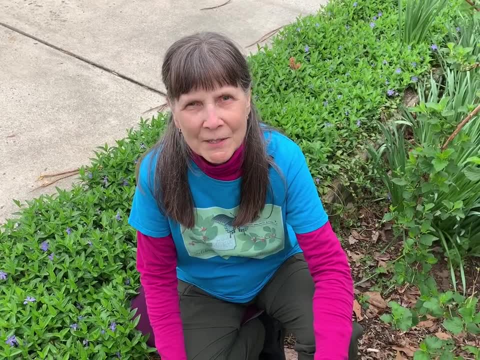 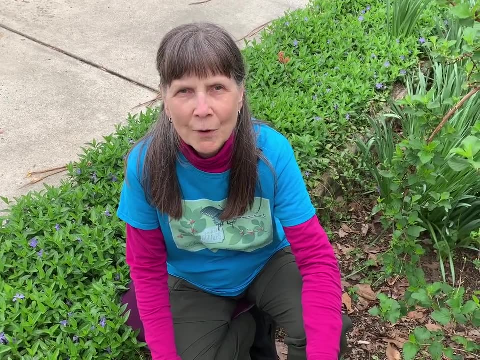 Periwinkle has all the characteristics of invasiveness. First of all, it's not native to the United States. It was introduced here in the 1700s from the Mediterranean region. Secondly, the plant doesn't necessarily remain where it was planted. 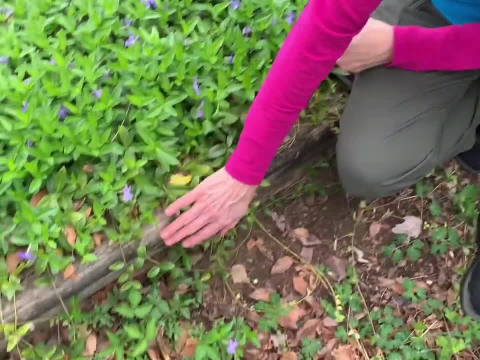 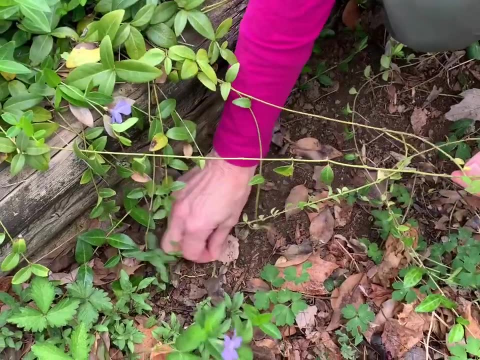 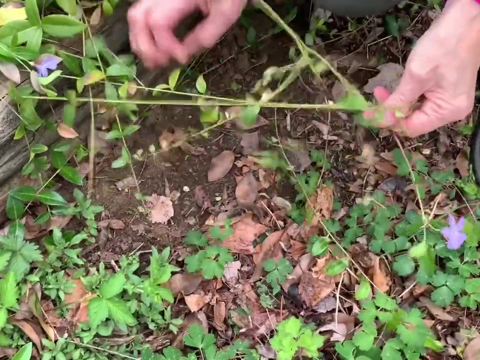 This bed in my neighbor's yard is now sending out these above-ground runners, these stolons that are reaching out, and then sending out little additional roots to introduce new plants that will be spreading And if I don't keep this under control, this could easily spread six feet well onto my property. 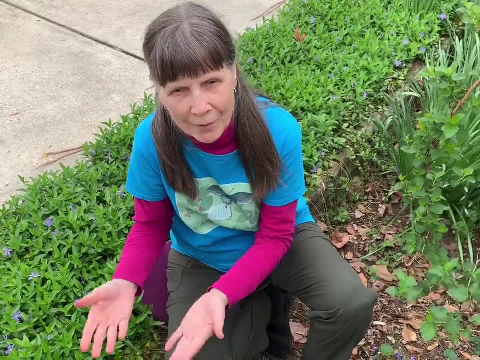 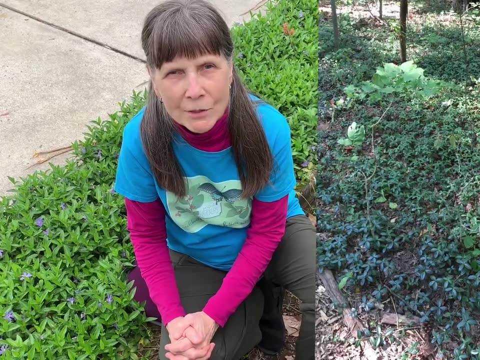 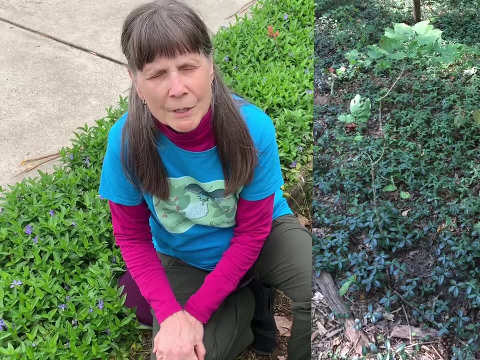 What's even of greatest concern, however, is what happens when this occurs. this vegetative spread in our natural areas. Periwinkle can grow in dense shade, and that means that it can spread rampantly in the undergrowth of our forests, suppressing the native herbaceous vegetation. 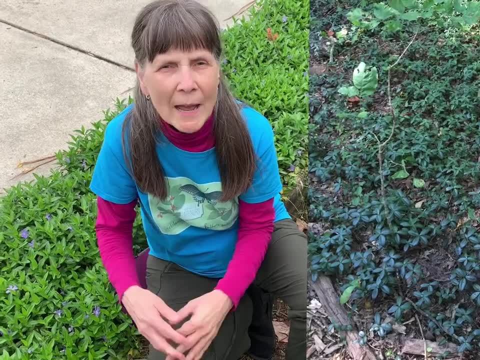 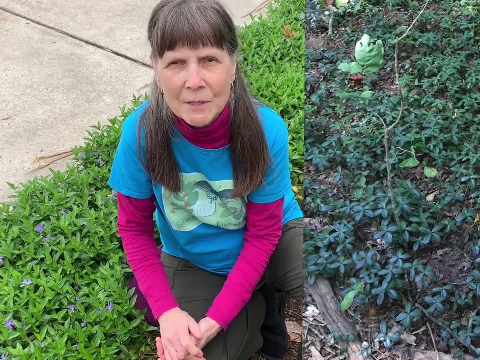 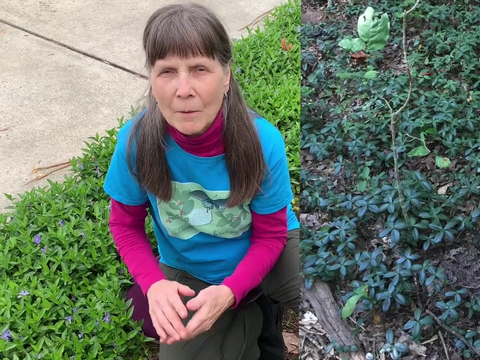 Secondly, it can inhibit the natural succession process in the forest by preventing the successful growth of small saplings that would then grow up to become the new generation of trees. This process happens because the plant sends out chemicals. It's referred to as an acid. 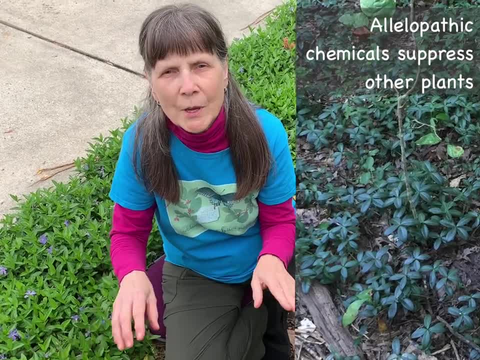 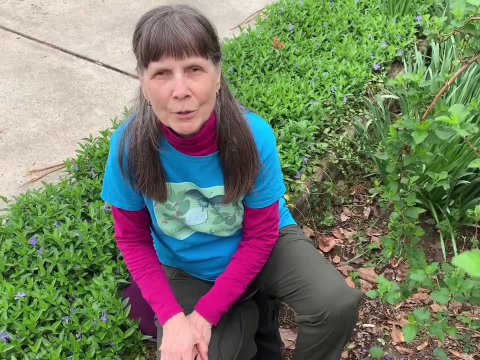 It's referred to as an acid. It's referred to as an acid. It's referred to as an allelopathic plant. It sends out chemicals to subdue the growth of other neighboring plants. Additionally, periwinkle does not provide any support to our local wildlife. 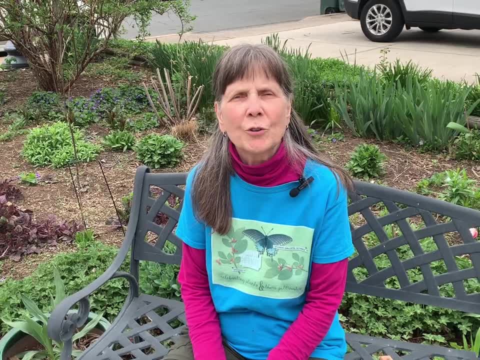 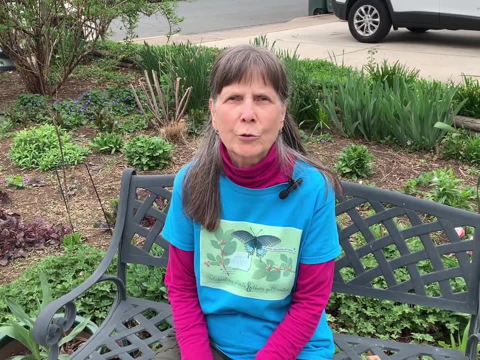 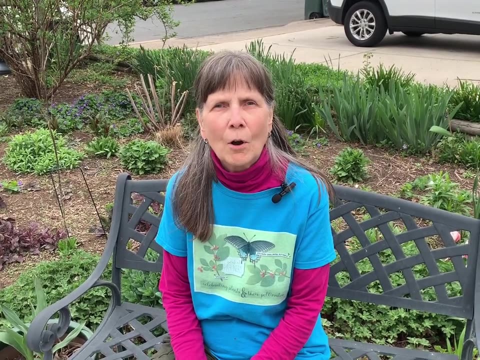 Despite being designated as invasive throughout the eastern United States, periwinkle is still widely advertised and easily available in the horticulture trade. You can learn about techniques for managing this plant under invasives. You can learn about techniques for managing this plant under invasives. 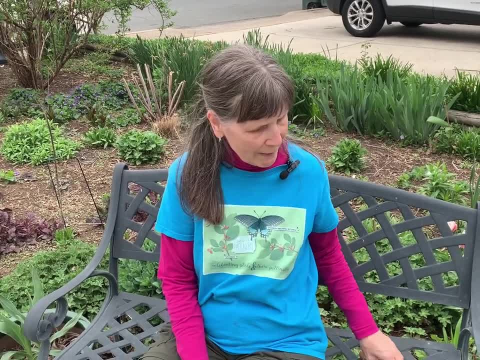 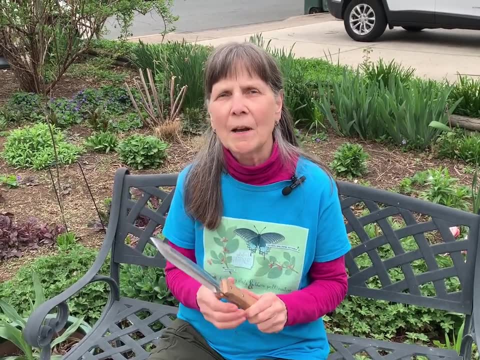 on our Master Gardeners of Northern Virginia website. I'd just like to mention that I like to use my favorite gardening tool, the hoary hoary knife, as an easy way to remove the little bits of vinca that you saw coming over from my neighbor's property. 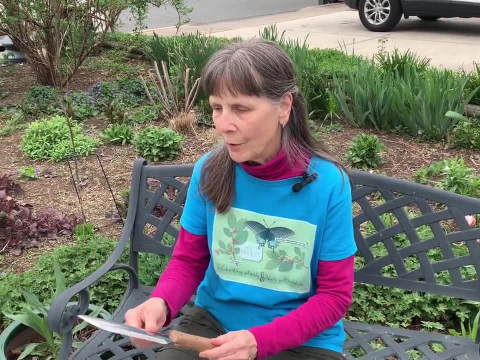 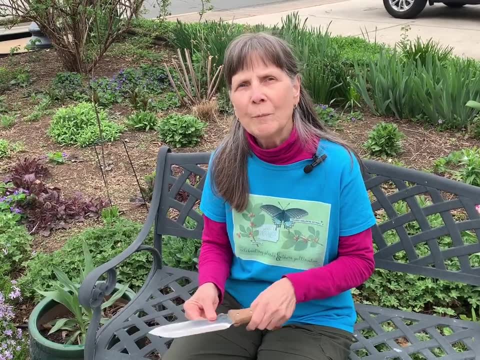 With this sharp pointed tip I can lift under those stolons, those above-ground stems and make sure that I'm getting all of those roots out completely. You want to make sure not to leave any fragments because those could reroute and then start the spreading process. 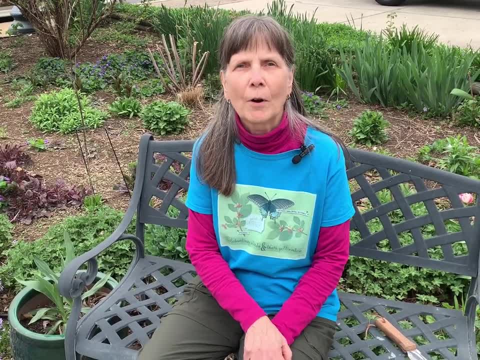 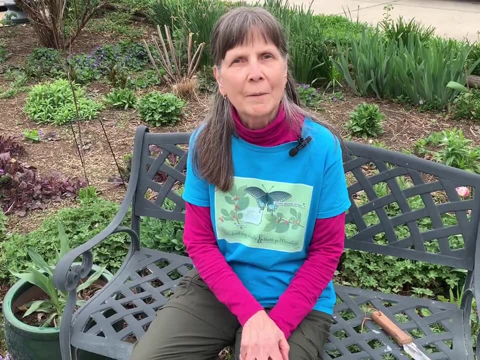 because those could reroute and then start the spreading process all over again. Luckily, there are a number of native brown covers that make fabulous replacements for periwinkle, and I'd like to introduce you to three of them that are here in my own garden. The first native brown cover that I'd like 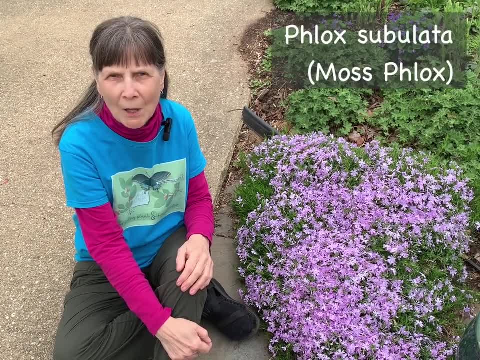 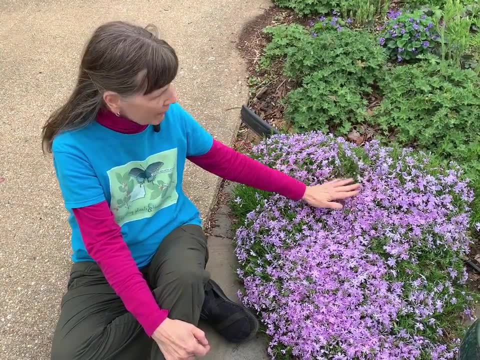 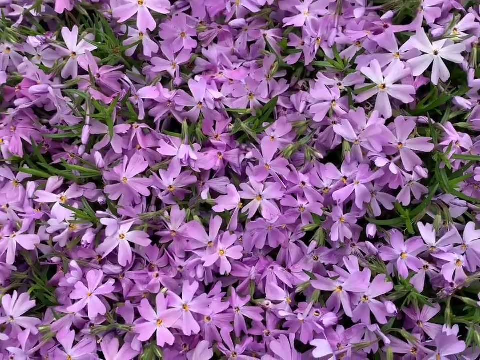 to suggest as a replacement is Moss Phlox, Phlox subulata. This plant right here is growing about six inches tall and you can see how nicely it spreads. It makes a very dense, weed-free mat. Moss Phlox has very soft, needle-like 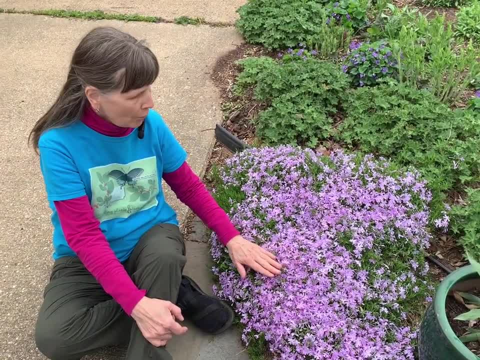 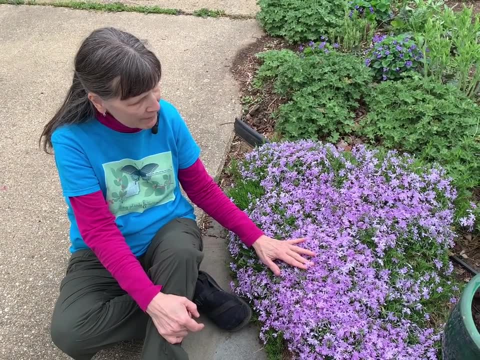 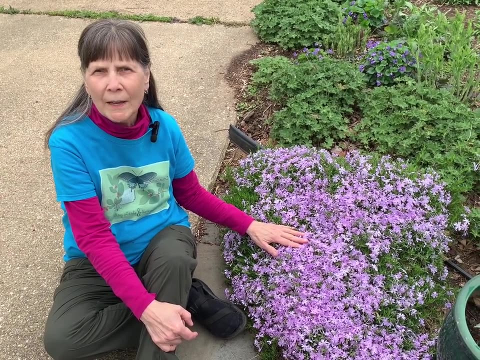 evergreen foliage and here in early April this plant is in already in full bloom. It has lovely tubular flowers with a slight fragrance that provide a wonderful early nectar source for our pollinators. Moss Phlox grows particularly well in full Sun. It's tolerant of dry and rocky soil. 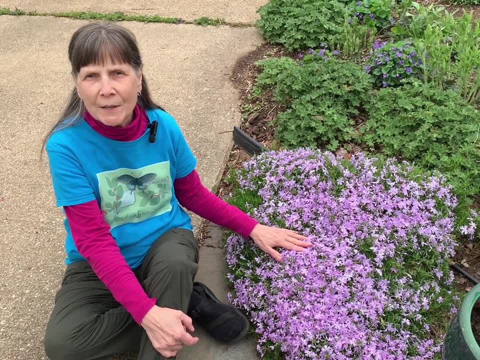 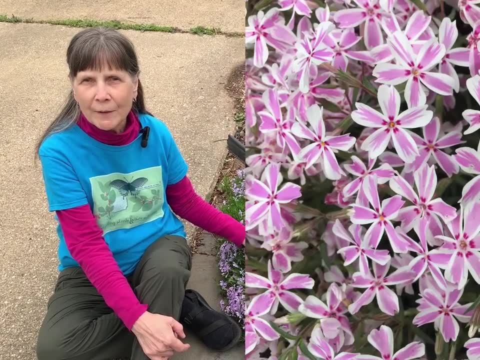 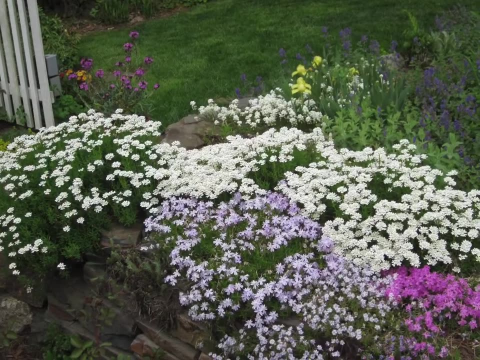 early summer and early fall. Moss Phlox is a very good choice for a urban pollution and even salt, which makes it ideal for planting along sidewalks and driveways. It also looks especially attractive in rock gardens and it's very effective when planted on slopes to control erosion. Luckily, Moss 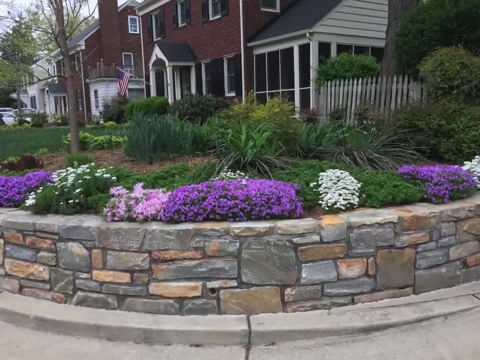 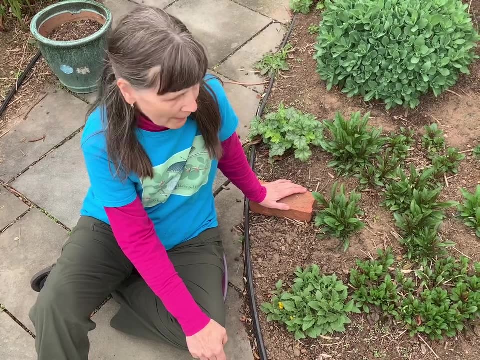 Phlox is available in many colors throughout the horticulture trade. You may not even have realized that it is a native plant. The second native ground cover here is Green and Blue Phlox, Phlox subulata. This plant is a very 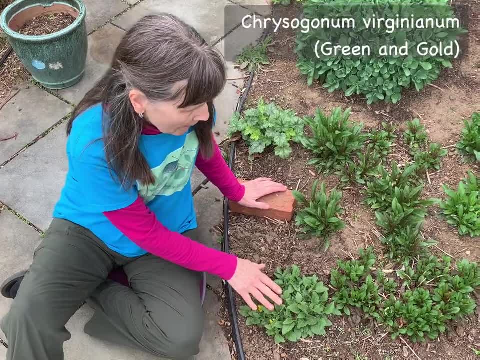 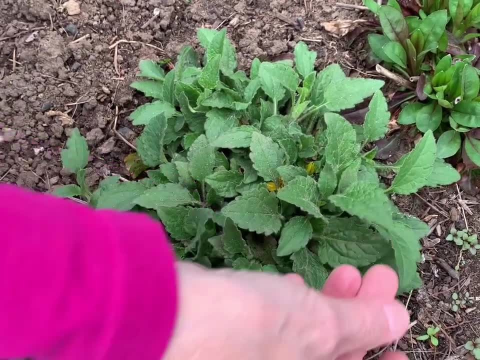 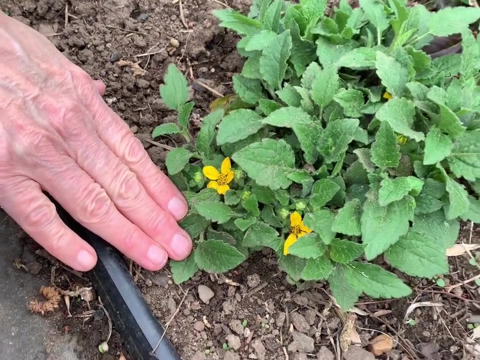 junto green and gold Chrysogonium virginienum, Another mat forming plant with dense foliage. This time the foliage is very velvety in texture. You can just see the beginnings of the little star-like yellow flowers. These will continue on for a month or so, and the plant can even bloom intermittently. 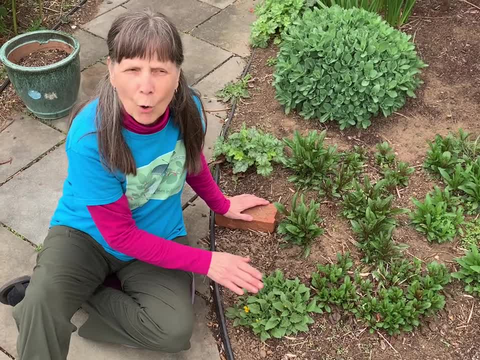